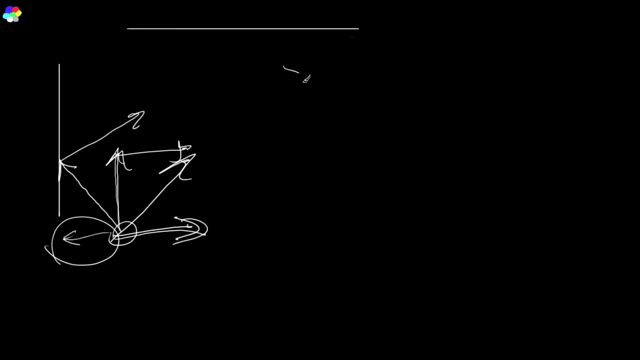 Now, what we want to do today Is: we want to do that same thing, but we want to be able to calculate the velocity here with an arbitrary inclination of our wall. And what people will often do when confronted with a problem like this is, they'll say: 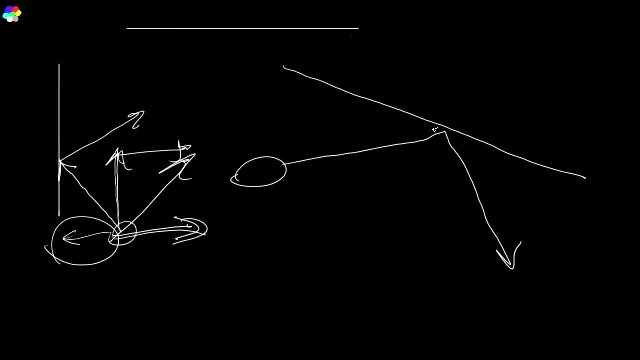 Well, okay, I know what reflection, how it works. This angle is going to be equal to this angle. So all I've got to do is, you know like I guess, calculate this angle and then this angle, And then I can get this angle the same, and then I just have to use some trigonometry to figure out this vector. 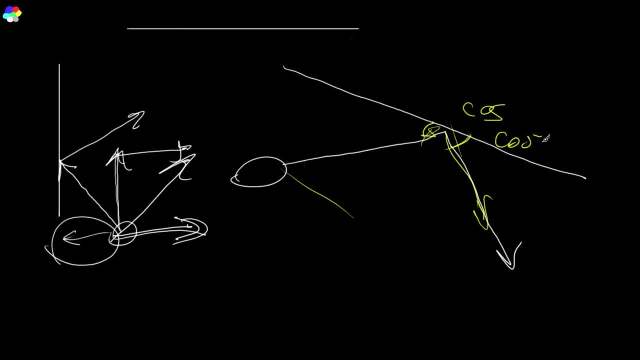 And you're doing a lot of cos and a lot of you know like cos negative one or sine negative one or whatever, And it's not so. It's complicated but it's not the hardest. But the real bad thing is that these operations are incredibly slow to do on a computer. 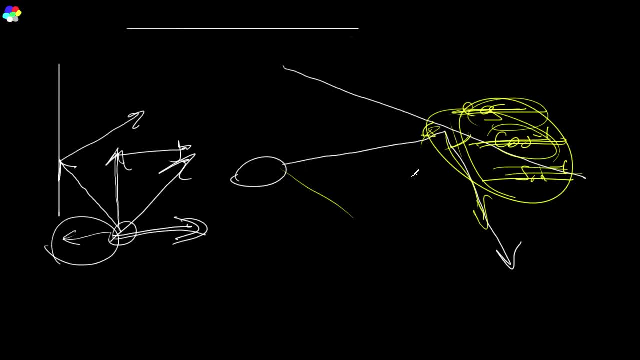 So we would like to avoid them if possible. And what happens when you use Vectors and dot products to calculate this instead of angles is you don't have to use any cosine sign, none of this stuff. You do it with a few simple multiplications and addition, subtraction. it's super fast. 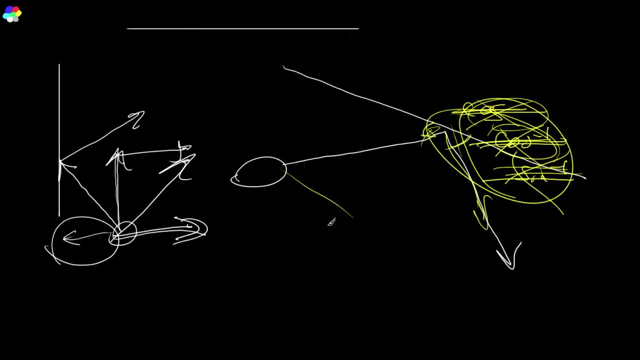 And it's a real. It's a different way of looking at the problem And it can be much cleaner to solve a problem with vector operations instead of with angles. So, now that I've set the stage, what the hell is a dot product? 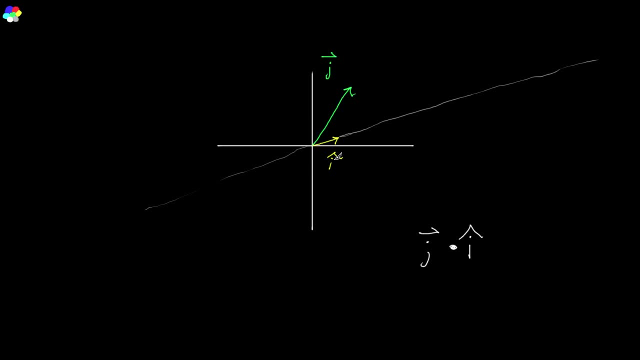 Alright, let's take two vectors here: J And I Hat And uh the hat here. when you put a hat on a vector, that means that the vector has a length of one, so it's a normalized vector. 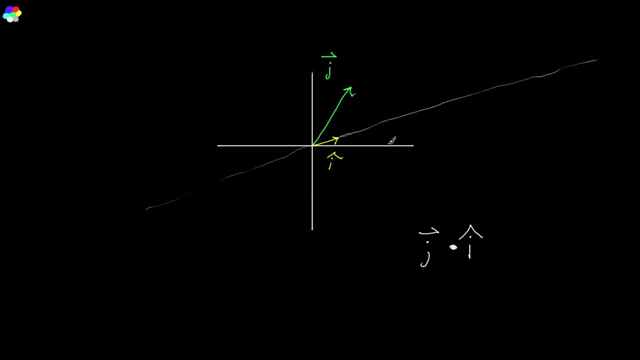 So we want to calculate JIHat. How do we do that? Well, first step, we want to visualize this. Let's draw a line that is in the same direction as IHat. So this is the line of IHat. we'll call this. 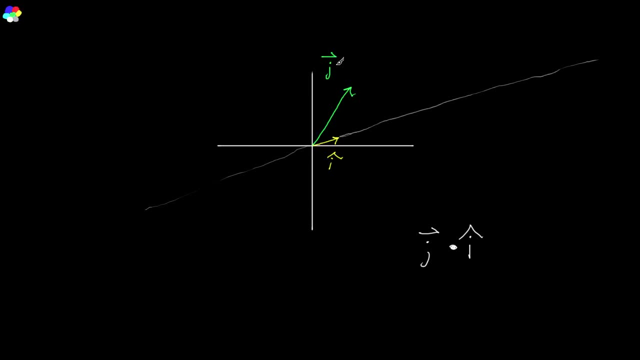 And to calculate the dot product. what we're going to do is we're going to project J onto this line. What does that mean? Well, it means we're going to draw a line from the tip of J Down to the line of IHat. 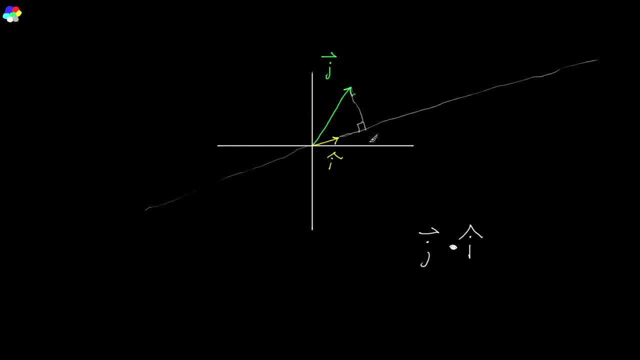 And we're going to draw it such that the angle is 90 degrees And this gives us the projection of J in the line of IHat. Okay, Pretty simple to visualize right Now the length Of this projection here. 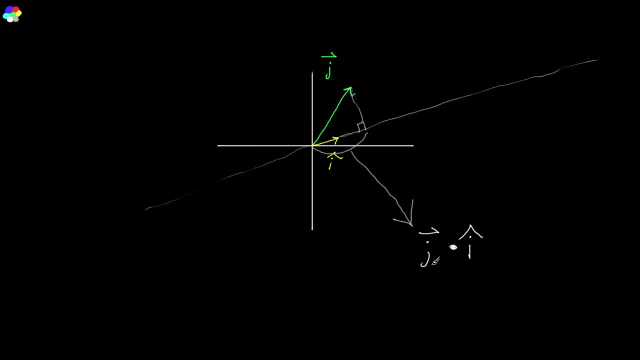 That is just exactly JIHat. So the dot product, it just gives us the length of the projection of J into IHat. And one thing you notice about this is very interesting: Dot product is operation between two vectors, but it yields a scalar value. 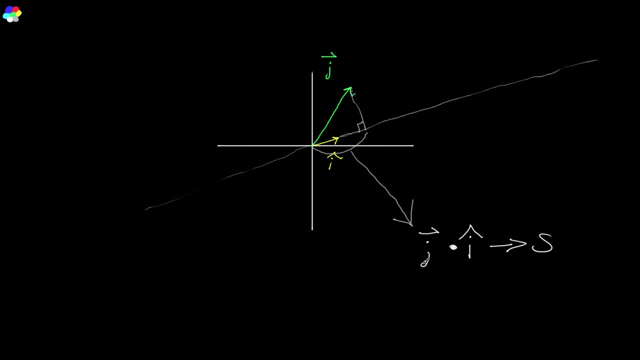 So that's the first thing to know about dot product. It's a vector operation that yields a scalar Interesting. Some other things to note is basically what this is doing is. this is giving us How much of J is going in the direction of I. 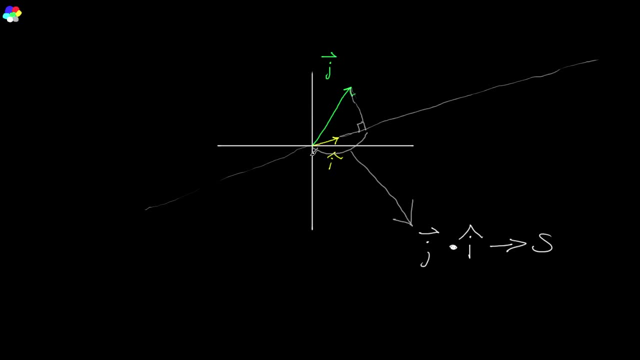 Okay. So if we look at a different vector here, Let's take a look at a vector. We'll call this one. We'll call this one K. Alright. Now if we do KIHat, What do you think the value is going to be for this? 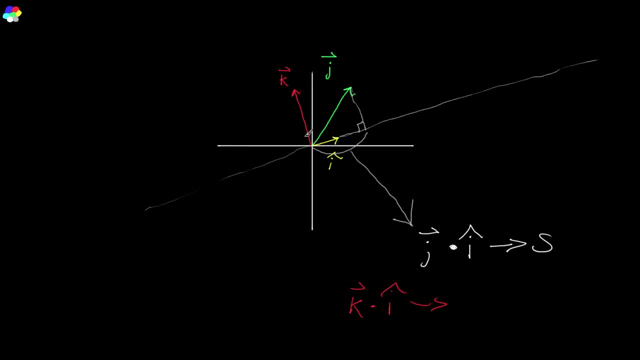 Well, if we project this down 90 degrees, K is already 90 degrees to I, So the projection is just going to be right at the origin. The length of that line segment is 0. So we can see that things that are perpendicular to I. 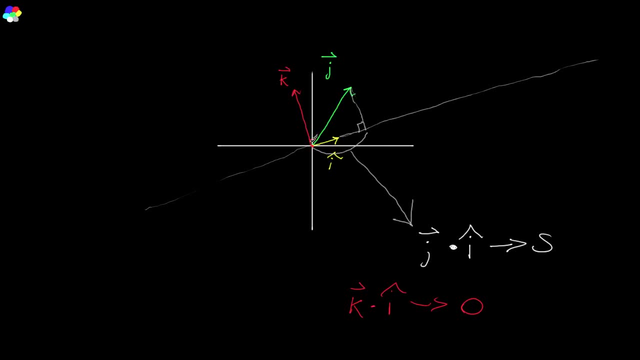 The dot with them is going to be 0.. Because none of this is going in the direction of I. It's all going orthogonal to I Or perpendicular to I. None of it is going in this direction, So the answer is 0. 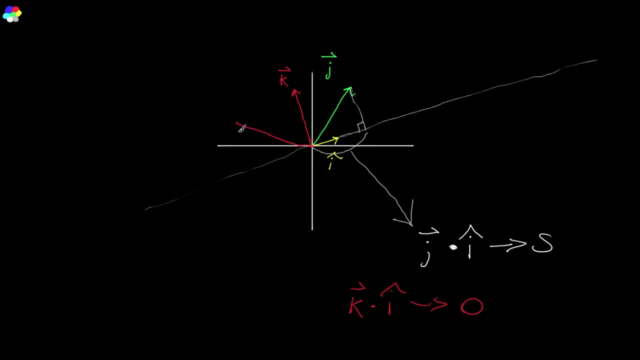 Likewise, if we put a vector going in this direction here- I don't know, I'll just call this one MHat M, What do you think the dot product is going to be? Well, It's going to be this length here. 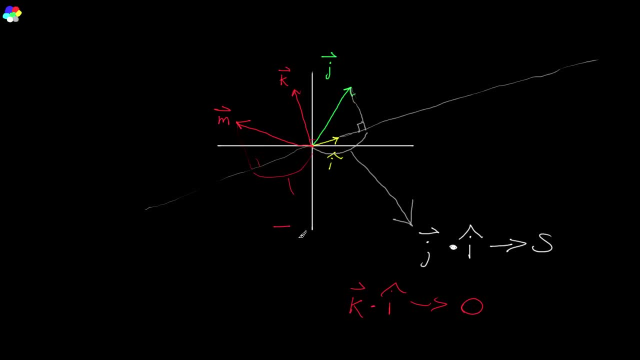 Whatever that is, But it's going to be negative, Negative length Because it's going in the opposite direction of I. So the dot product tells us how much we're going in the direction, Or in the opposite direction Or not at all. 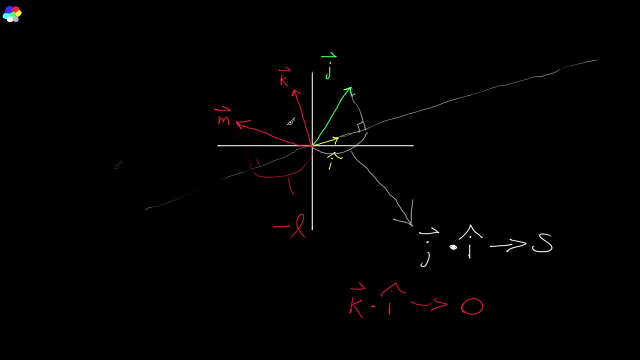 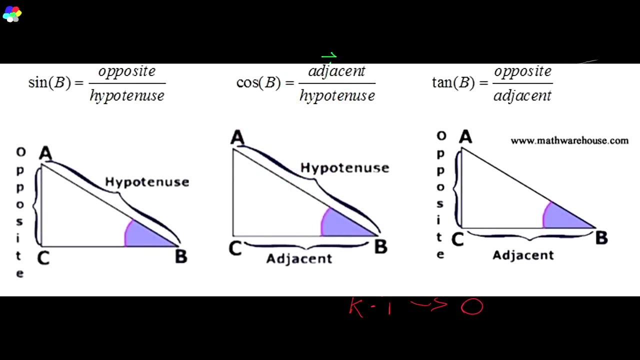 It's very important information. So the next question is: How do we actually calculate this dot product here Mathematically? Well, If we know this angle here, Theta, Then we could use SOHCAHTOA to calculate that. 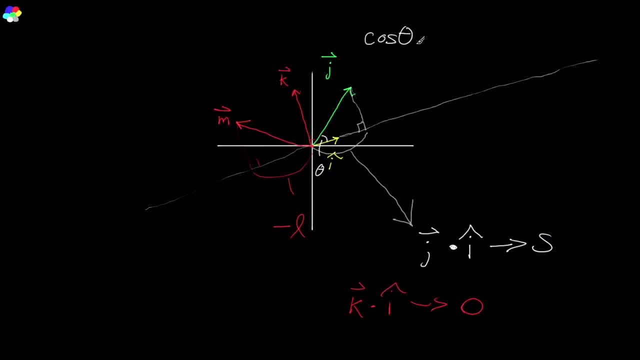 So SOHCAHTOA tells us that Cos theta is equal to the adjacent over the hypotenuse, So we want to know the adjacent, That's this one, The side that's adjacent to theta, And we know the hypotenuse. 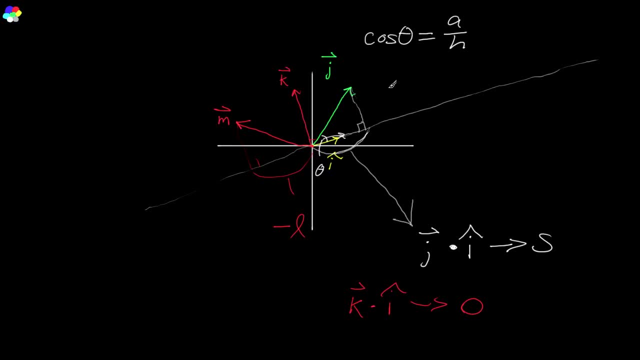 That's just the length of J, And we know theta, So we should be able to calculate this. So the hypotenuse is equal to the length of J. So if we do a little bit of algebra We know A. 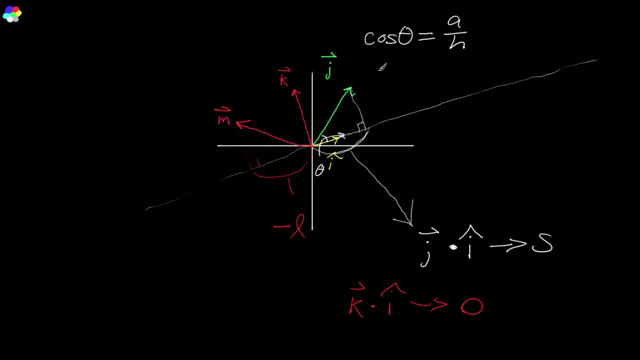 Which is equal to the dot product. So we can do J. J dot I hat, Which is just A, Is equal to H, Which is just the length of J Times Cos theta. And there you go. So your dot product is just the length of J. 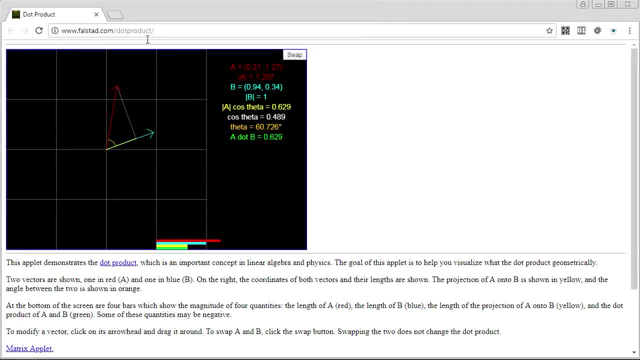 Times cos theta. So let's take a look at this demonstration applet here. You can check it out at this address. So we've got two vectors, A and B. B is a length of 1.. So that's our unit vector. 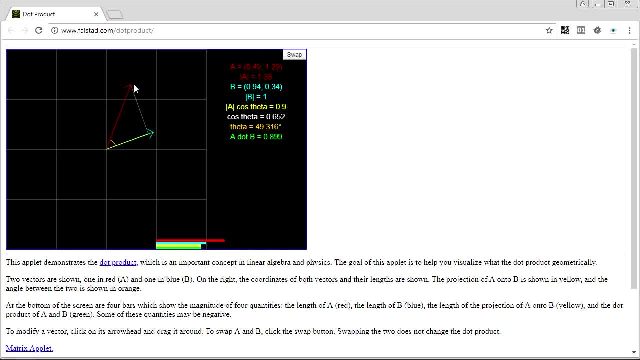 Our normalized vector. And then I'm moving A around And you can see here The yellow line gives us the projection of A in the line of B, And we can see here The calculation for that is A cos theta. And we can see that our applet is telling us that that's equal to A dot B. 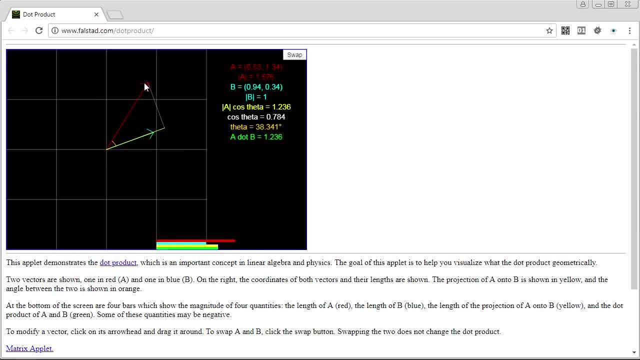 Very interesting. Now, up until now, All we've been doing- Here we can see a negative, Here we can see it goes down to 0.. Now, up until now, What we've been doing is We have been having one vector, that's free. 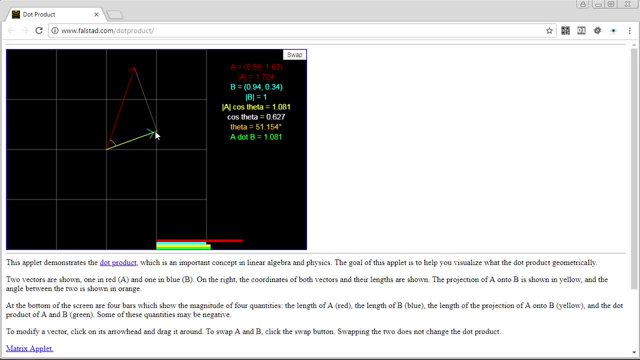 But the other vector has to have a length of 1.. But what if this vector had a length that wasn't unit length? How does that affect the result of A dot B? Well, let's scale B up, Let's double its length. 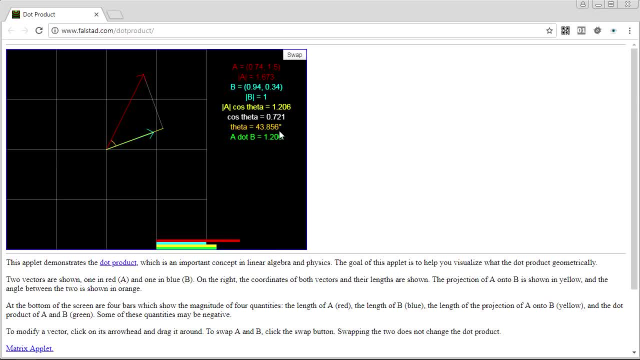 And see what happens to A dot B. So we want to keep the same angle, 43.8 degrees about, But we want to make the length of B twice as long, So let me do that. So here I've doubled the length of B about. 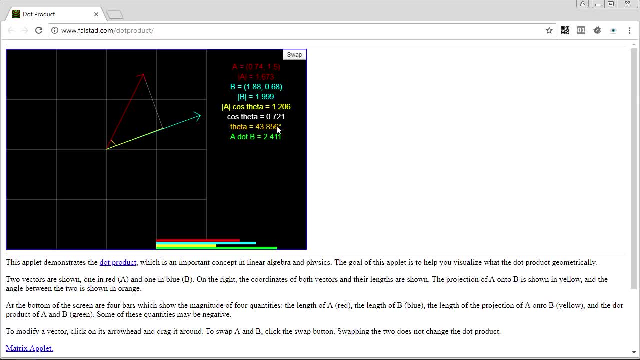 While keeping the angle Right. about the same. And if we look at A dot B, It has doubled. So the length of the projection is still 1.2.. That doesn't change. But A dot B doubles when you double the length of B. 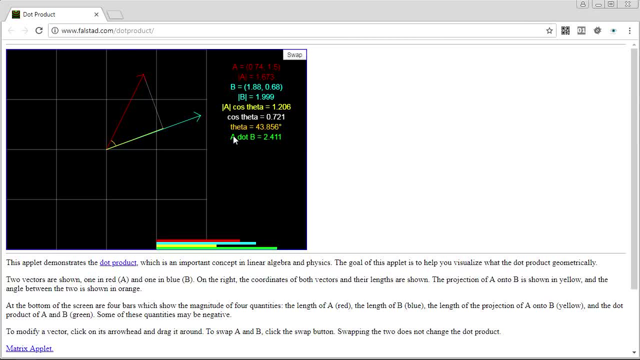 So what is the actual formula for the dot product then? Because it's not just dependent on the length of A, It also depends on the length of B, And the answer is quite simple For any two arbitrary vectors That both have any kind of length you want. 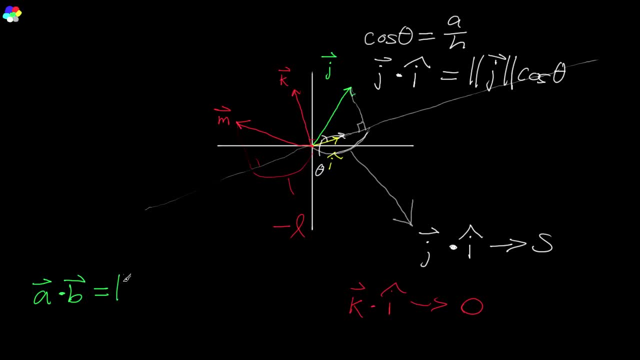 The dot product is just going to be the length of A Times the length of B Times cos theta, Because if you double the length of B, The dot product doubles. If you double the length of A, The dot product doubles. So it's the product of their lengths. 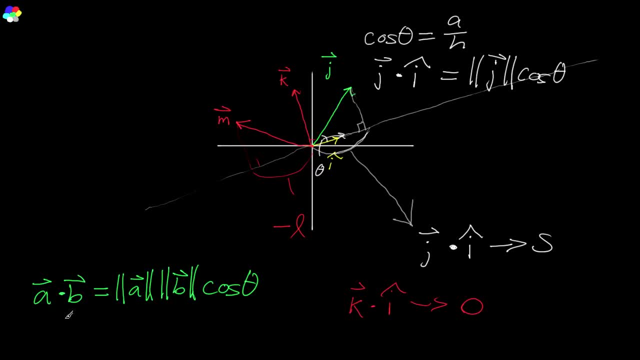 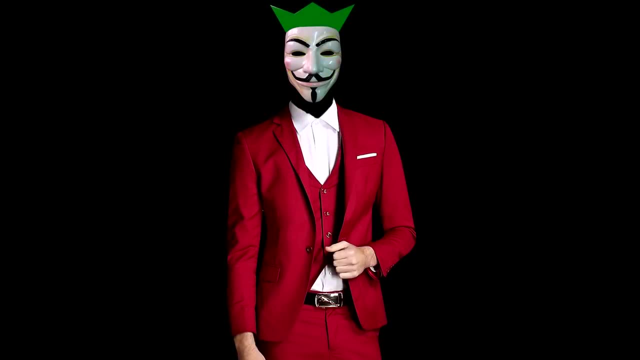 Times the cos of the angle between them. And this is the angle version Of the dot product formula. Now you might be saying, Chili, I don't get the big deal here. You said that we could do our bullshits. 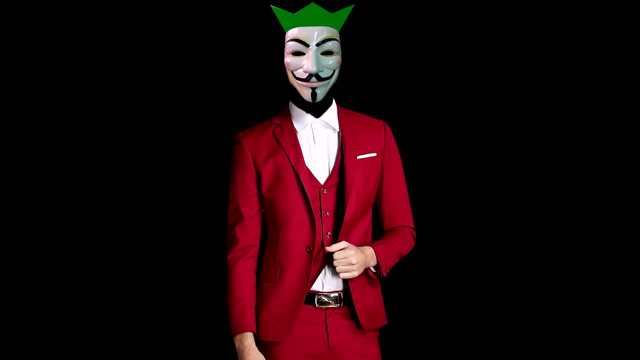 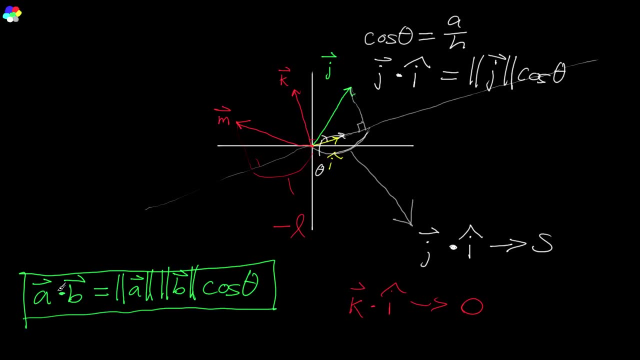 Without having to use cos and sine. But now you've done a big cos and sine in here. Well, here's the deal. There's another way to calculate the dot product. It gives you the exact same answer, But that doesn't use trigonometry. 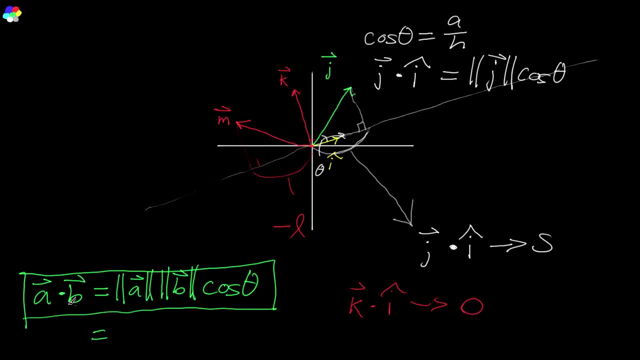 And it's very simple. Let's say A and B are two dimensional vectors, The dot product is going to be AX Times, BX Plus AY Times, BY. And there you go. It's that simple, And this will give you the same result. 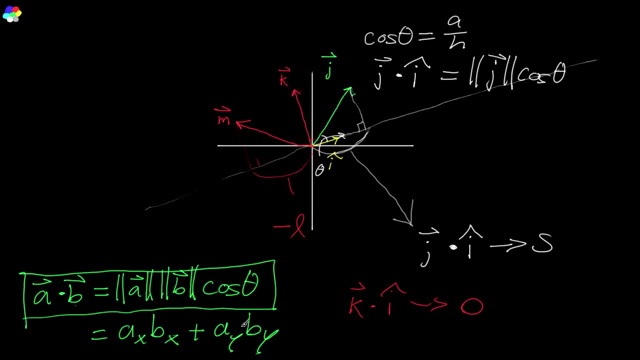 As this complicated thing here. But it's very simple. It's just a couple multiplies and an add And that's all you need, And you can solve complicated problems That require, That conceptually require angles, Without needing to know the angles. 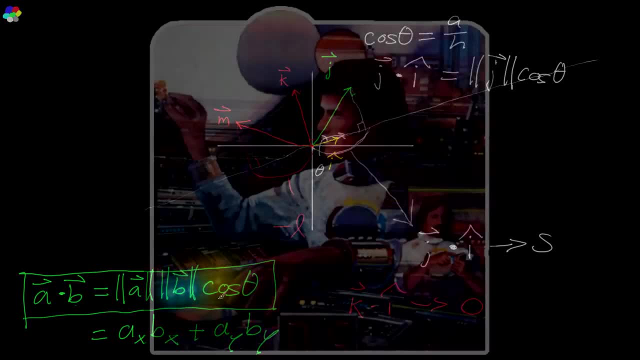 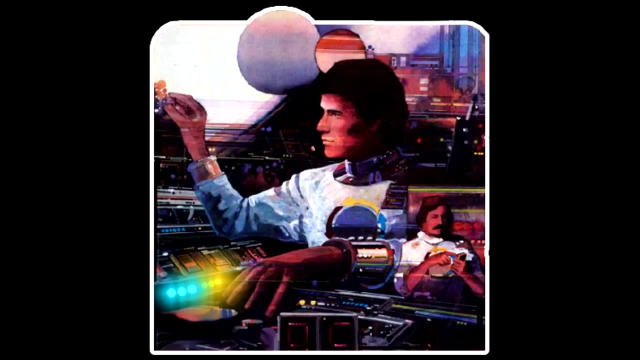 You solve them only knowing The components of the vectors, And that is incredibly powerful. This power of the dot product Allows you to think in terms of vectors And to diagram out your problems And solve them Without ever needing to worry about angles. 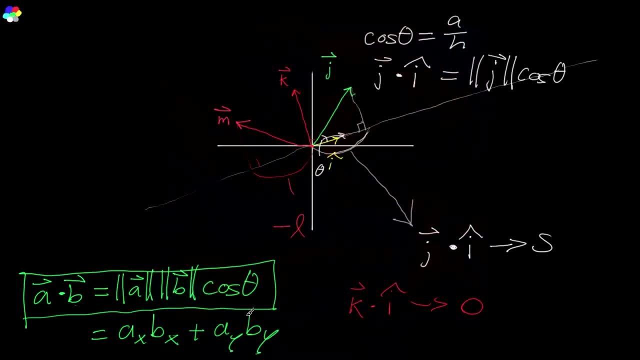 And also what you can do. Sometimes you might derive a problem And it has angles in cos When you derive out its formula And you can rework the formula And then substitute in the dot product Instead of these cos and sine. 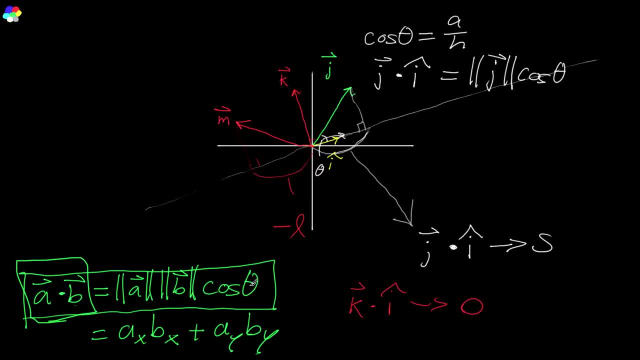 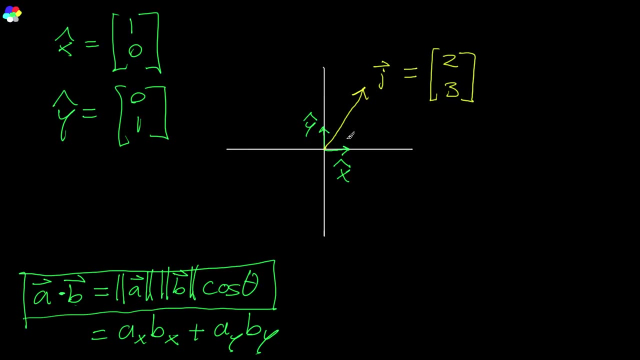 And theta, And you'll see me doing that In 3D fundamentals, But today We're going to work purely in vectors To solve the physics problem. Now, one of the most common uses That I have for dot product Is to figure out. 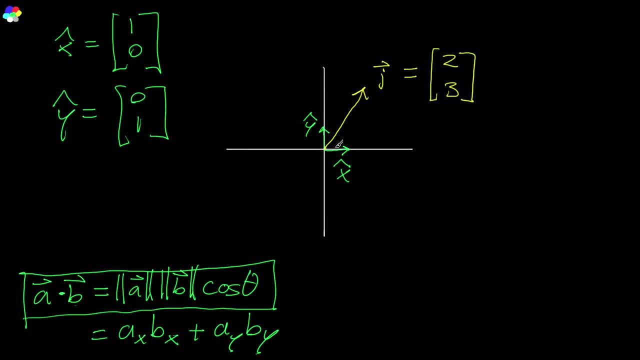 How much of one vector Is going in a certain direction. So the way we do that Is we define our direction With a unit vector in that direction. So let's define some basic ones. So y hat will be The unit vector going in the y axis. 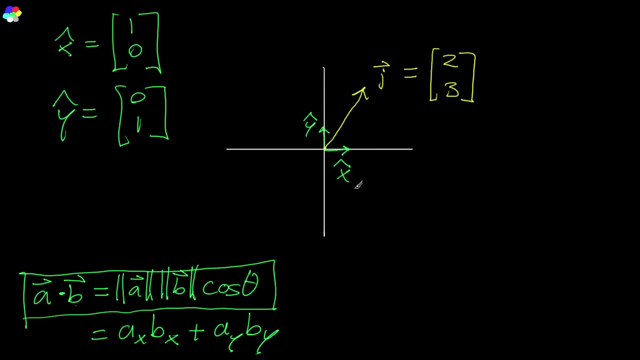 And x hat Will be the unit vector going in the x axis. And let's say we want to know how much of j Is going in the x direction. Well, we could just do. You know, j Dot, x hat Is equal to. 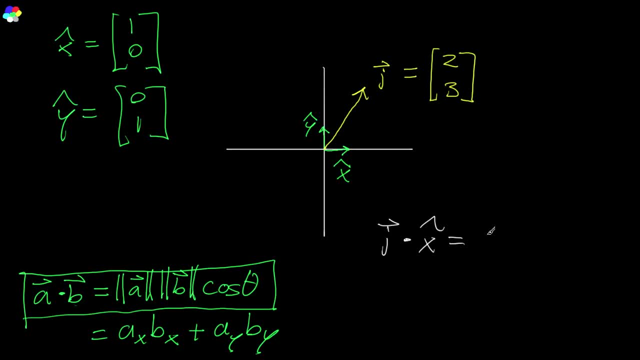 And here x is One zero. So we're going to do: Let's see here Two times one, Three Times zero, And that will Cancel out the y component And we're just left with two. So here we can dot product with x hat. 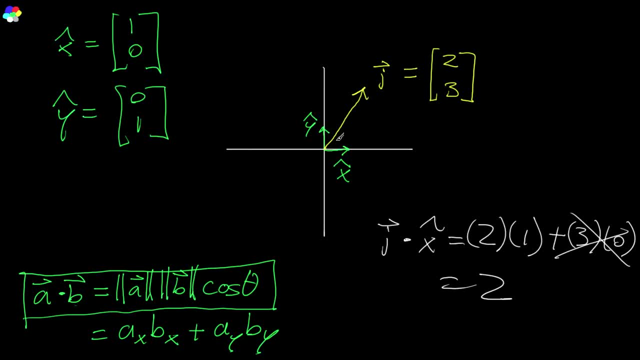 To get the x component. We could dot product with y hat To get the y component. You might be saying Whoopty, freaking, do chili. We could just look at the actual components of the vector And get the x component of the y component. 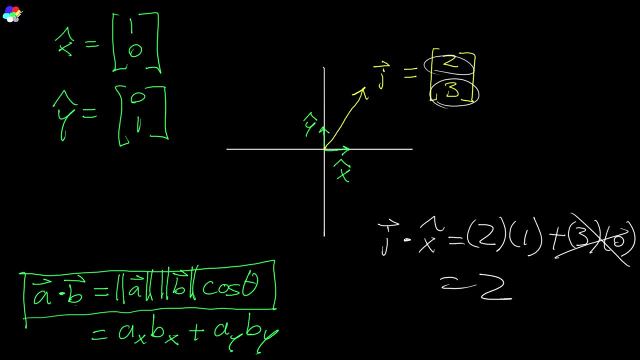 We don't need to do this song and dance, And you're correct, We can do another vector, Unit vector That's in an arbitrary direction Here. We'll call this one K hat, And we want to know how much of j hat. 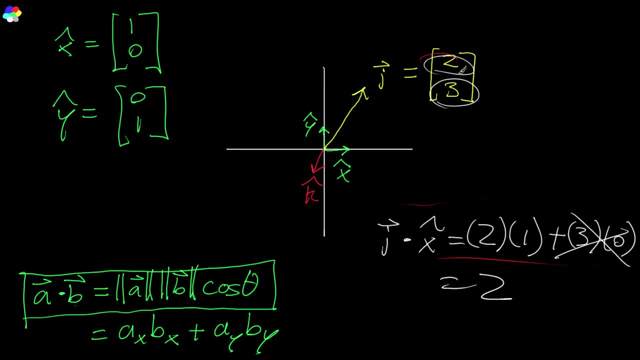 Is going in the direction of k hat And this will let us do it. You can't inspect it, You can't just look at the numbers here and tell, But with the dot product You get that information super easy. So it's very common to dot one vector. 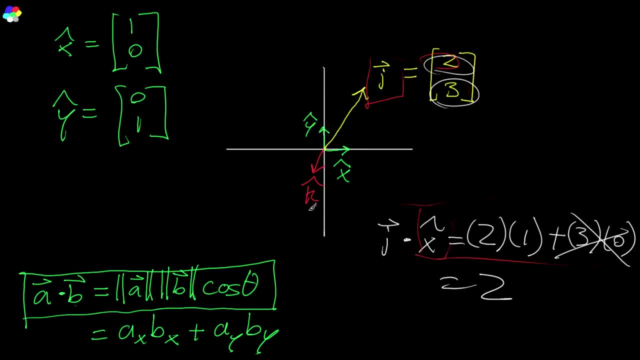 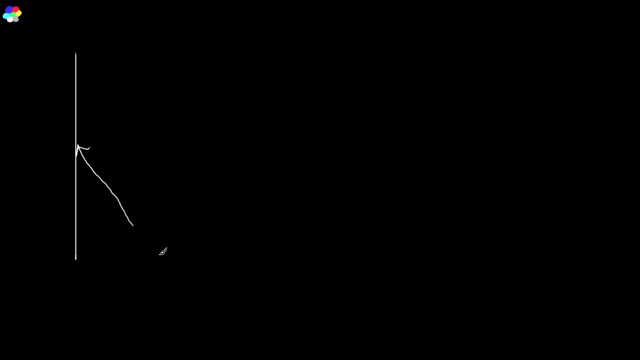 With a unit vector Of length, component Very common. So now let's use this information, This technology, And solve the problem of a ball Rebounding off of a wall That has an arbitrary inclination. So quick recap Of what we did in the fardenoid. 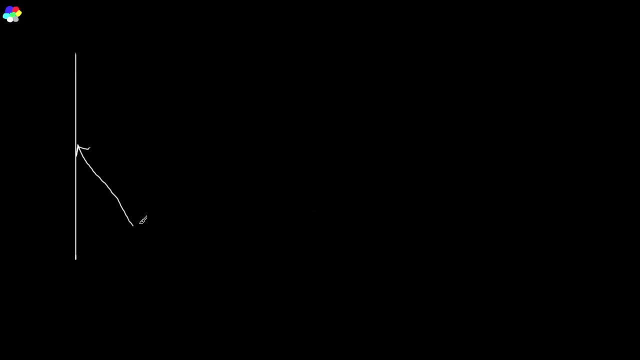 We had a ball. It was hitting the wall At a certain velocity And to rebound it, Basically we just flipped The component of the velocity That was going into the wall. So if the wall was vertical, The component into the wall is the x component. 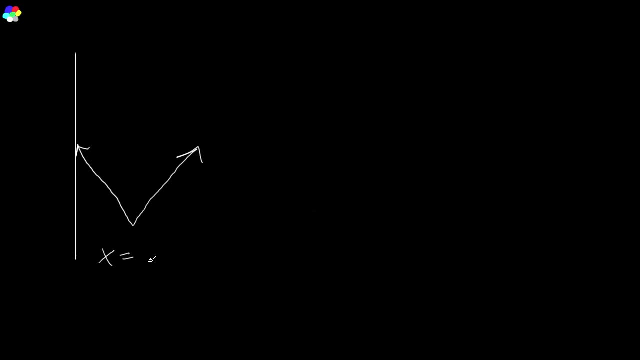 So we just do: x is equal to negative x. You know, x is equal to negative x there. You flip that And this is now the velocity That the ball is going to Rebound off the wall with. So it's very simple. 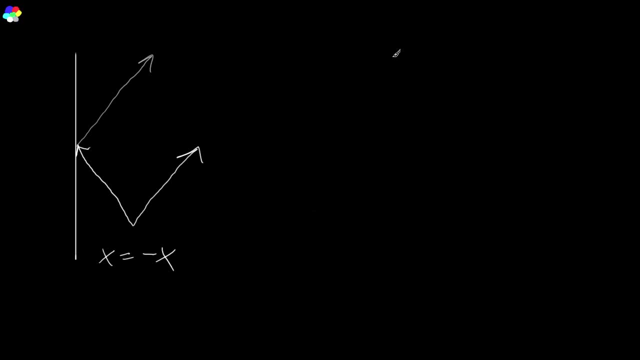 And we want to do the same thing. With our arbitrary inclination, We want to flip the part of the vector That is going into the wall. So first we have to calculate, Well, what part of the vector Is going into the wall? 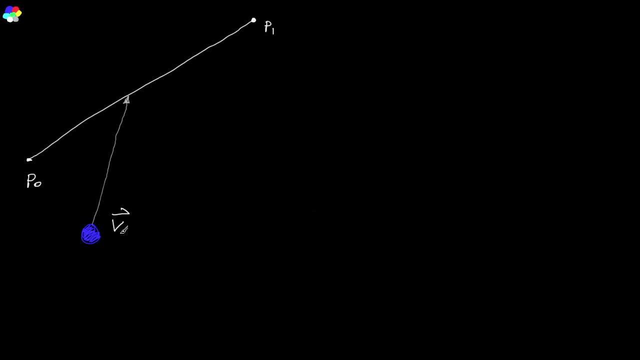 So let's do this step by step. So, basic setup with relevant information. We've got a ball. It's going towards the wall. It's got a velocity. The wall is defined by two points: P0 and P1.. How do we start? 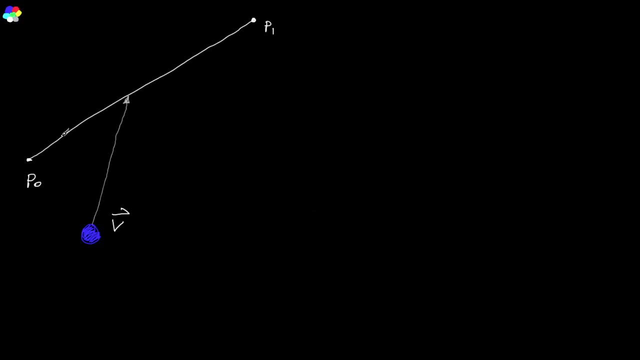 Well, let's get a vector That gives us the direction of the wall, And that vector Is just going to be, Let me see here, W, And W Is equal to P1 minus P0.. That gives us W. 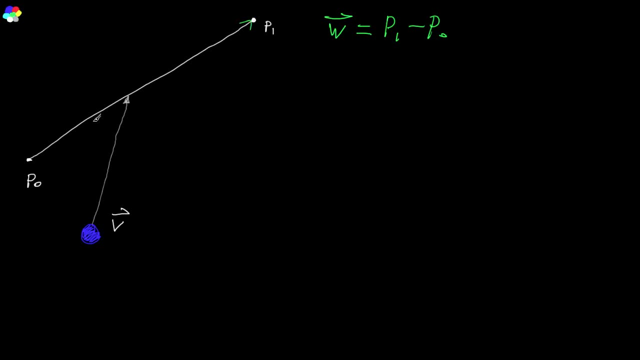 Which is going to be a vector that goes up to here. Now we want to get, Because the wall is going to be our direction, That we're going to be projecting onto, So we need a unit vector in that direction. That's simple. 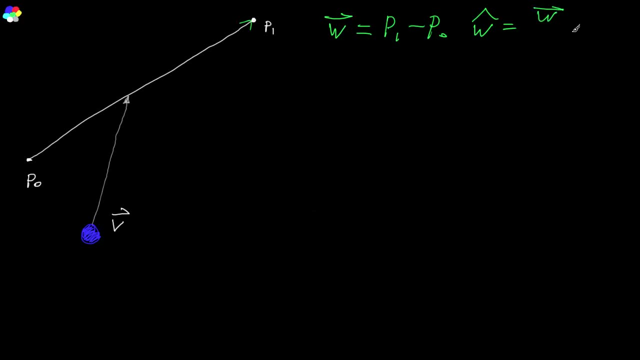 We'll call that. W hat Is equal to W divided by The length of W. So just normalizing W, That gives us W hat. So now we have W hat here. Good, Now let's get The amount of component. 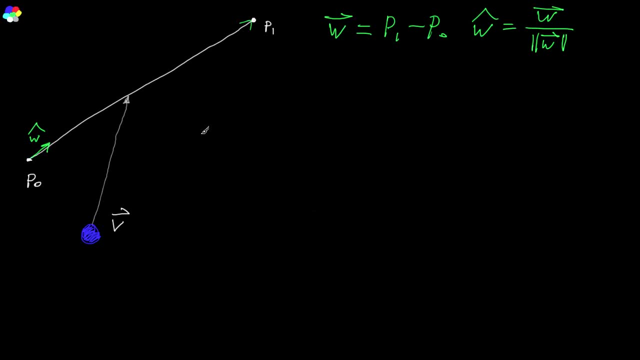 Of V That is going in the same direction As W. So to visualize that That's going to be, if this is V, That is going to be this projection here. So we calculate that With our good old friend That's going to be. 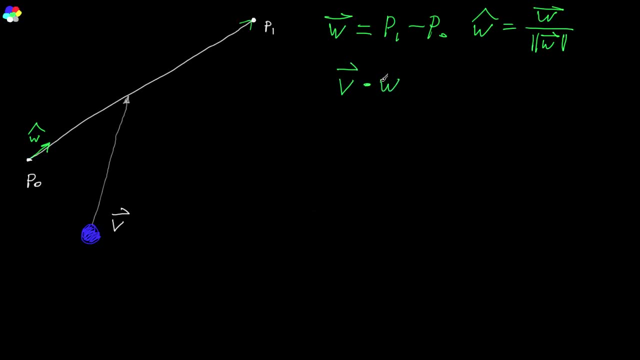 V Dot W hat. So that gives us the length of the projection In the direction of W, The length. But what I really want here Is I want the vector component In this direction. So I want a vector That has the length of the projection. 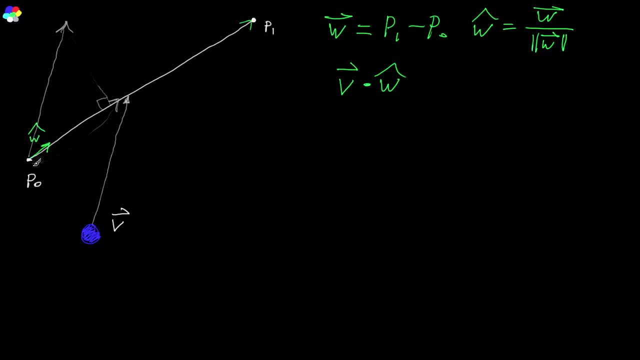 And is moving in the direction of W. So how do I do that? That has a length L In that direction. All I've got to do Is multiply By that unit vector, So this will give me The vector component. 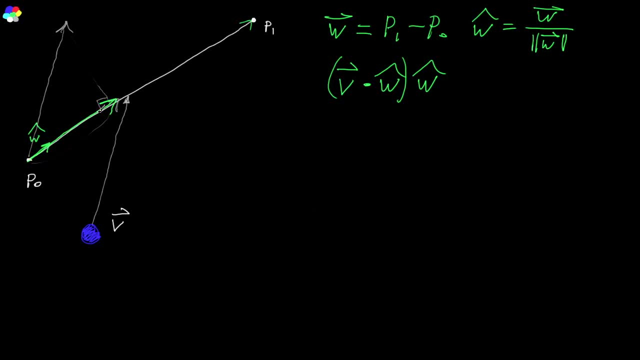 Of V That is going in the direction of W. That's the part of V, The vector part of V That is going in the direction of W, And let's call this K, for lack of a better, Better thing that I can think of. 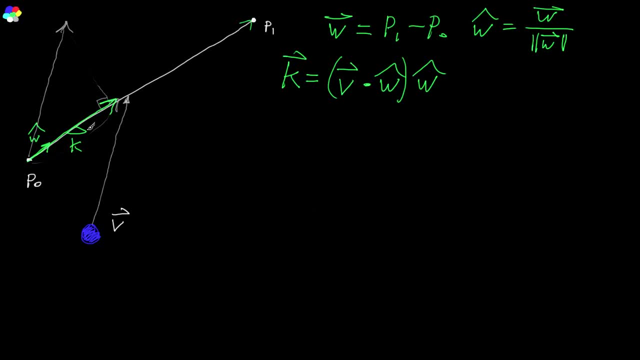 K is the part that is going in the direction Of the wall- The parallel component. But we want to know the part that is going Into the wall Right. That's the perpendicular component. Alright, So if we know the parallel component, 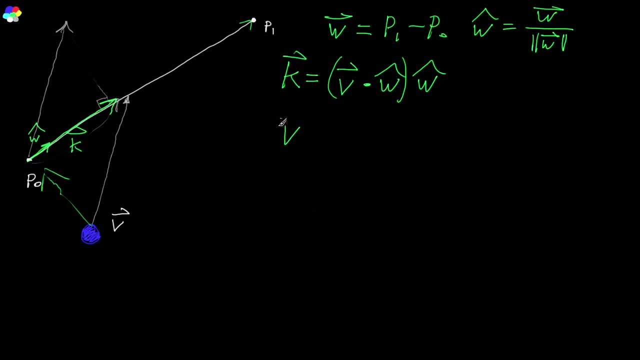 And we know the entire velocity. Velocity Is equal to the parallel component K Plus the perpendicular component J. So let's call this J For now. Now we know K, We know V, We don't know J, But we want to know J. 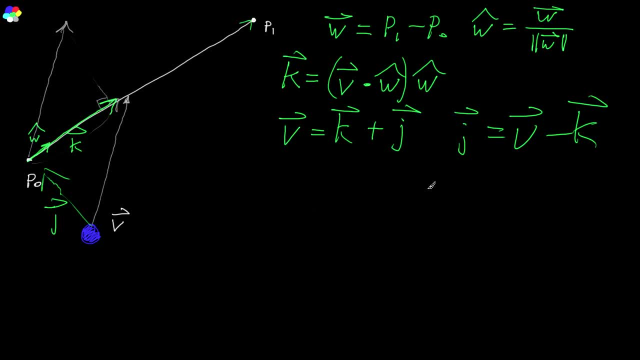 So it's just simple algebra: J is equal to V Minus K. Beautiful. So now we know the component Going into the wall. Now we want to flip that. How do we flip this component? Well, V Is equal to J. 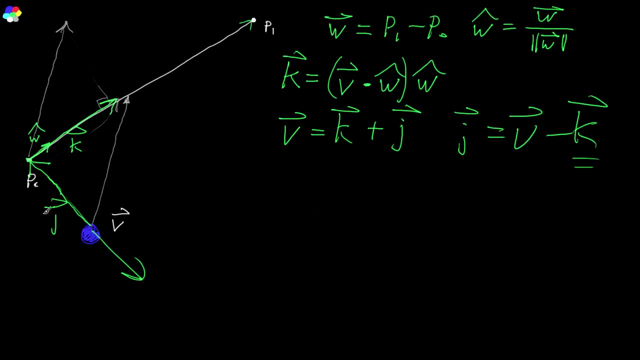 Plus K. If we add negative J To V, What happens? Well, adding negative J Will just cancel out the component Going into the wall, And now V will be running Exactly parallel to the wall. Stop that Now. if we add negative J, 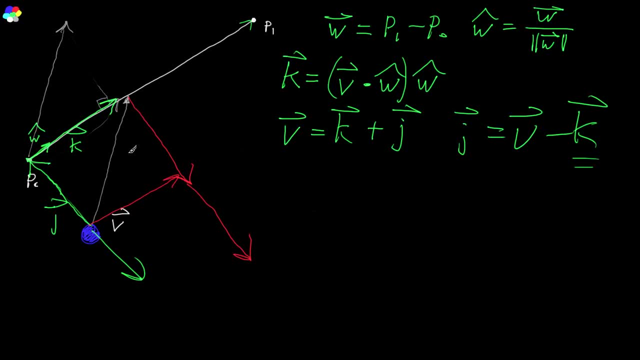 Times 2.. We'll actually be flipping V, Because adding once Negative J, once Subtracting J, Cancels it out, Subtracting it twice Flips it. And now V will be going in this direction, Which is the direction of rebound. 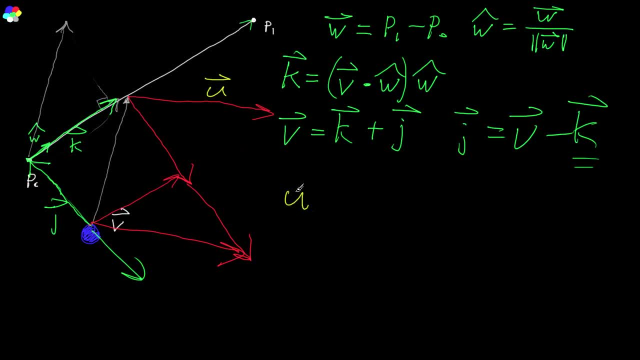 There you go, You've got the answer. So let's call the rebound vector here U. U is equal to V Minus 2.. Times J Is V Minus K. Okay, And that is V minus 2.. 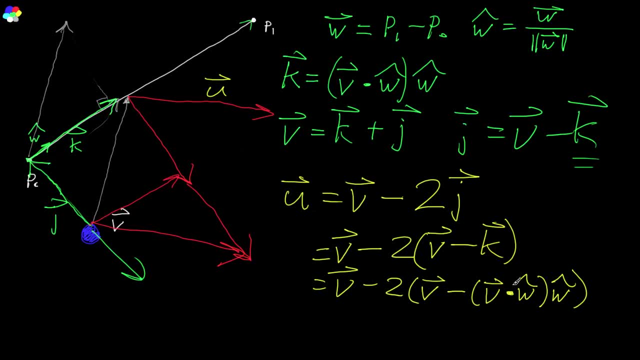 Times V minus V dot W Times W W hat. And we can simplify this a little bit: If we distribute this 2 here We get V minus 2 V Plus 2 times V dot W Times W hat. And so these guys you can just collect them together. 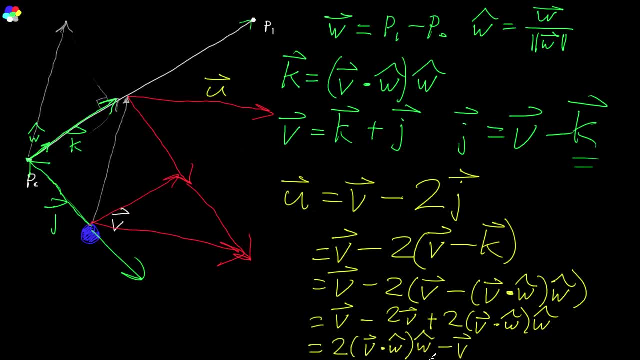 And you get W hat Times, W hat Minus V, And there you go. This is How you can calculate the rebound velocity, Dependent on the points of the wall And the initial velocity, And it's not a lot. 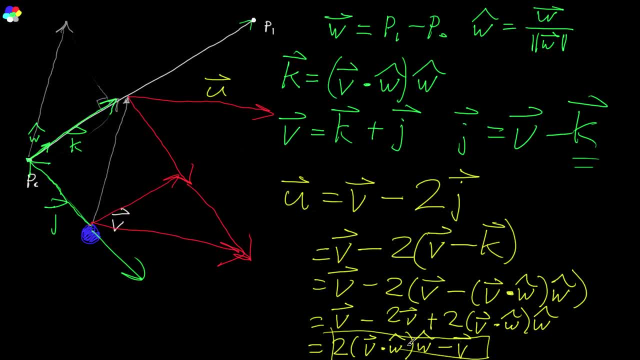 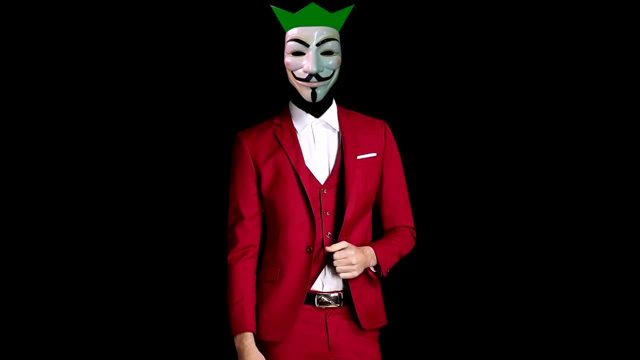 It's not a complicated operation For the computer to perform, It's just some multiplies, Some subtraction. It's very simple, Very straightforward, Easy to follow, Easy to visualize, Because it's a very visual thing with these vectors. But if you had trouble following,